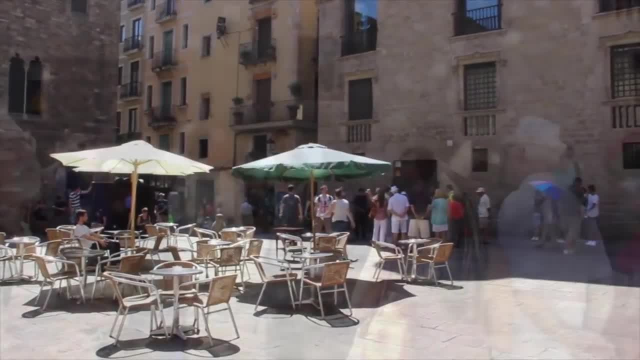 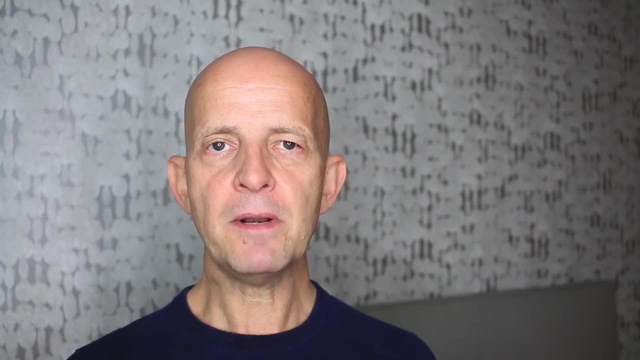 places like southern France, parts of Italy, the Balearic Islands, Sicily, Malta and, of course, parts of Spain like Barcelona. The second itinerary, and a very popular itinerary, is the Eastern Mediterranean. These tend to go from the beautiful city of Venice and then go down the 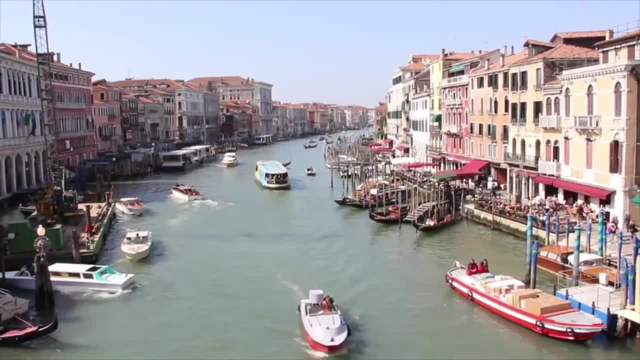 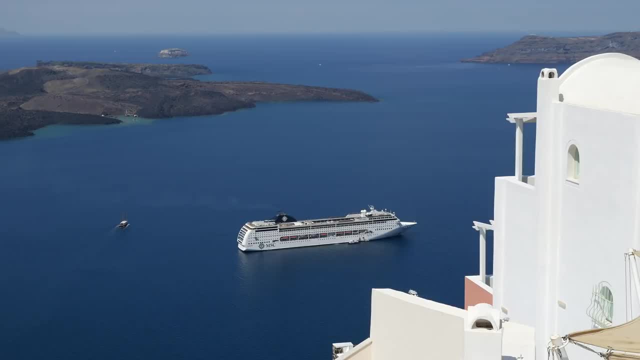 coast, So they include places like Croatia, Montenegro, Crete, Greece. The third very popular Mediterranean cruise is the Greek islands. This tends to be operated by cruise lines with smaller ships, which are more nifty for getting around the Greek islands. You then have the much longer 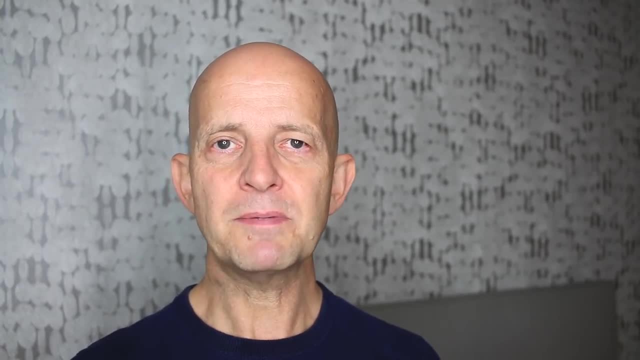 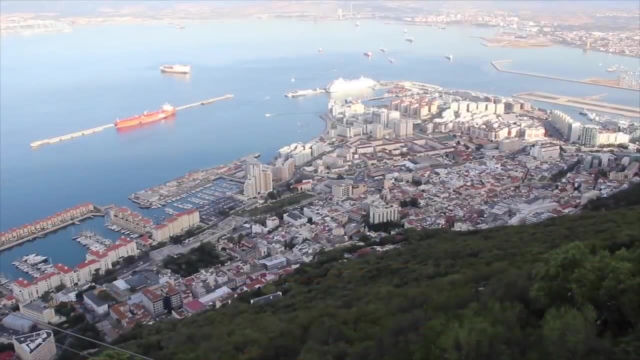 Mediterranean cruises, which can be up to two weeks long, and these are ones that particularly tend to go from more northern Europe. They might come from the UK or parts of northern Europe, and they will go to France, Portugal, Gibraltar, because they need to travel through that area before they. 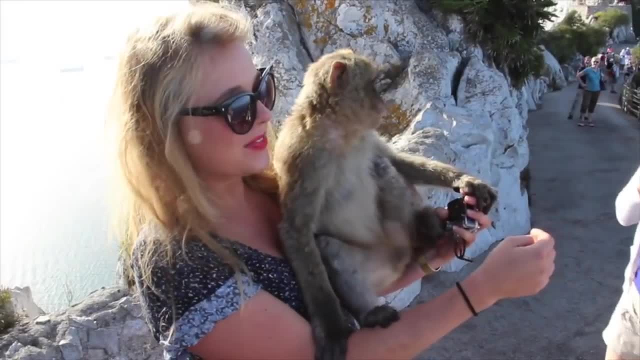 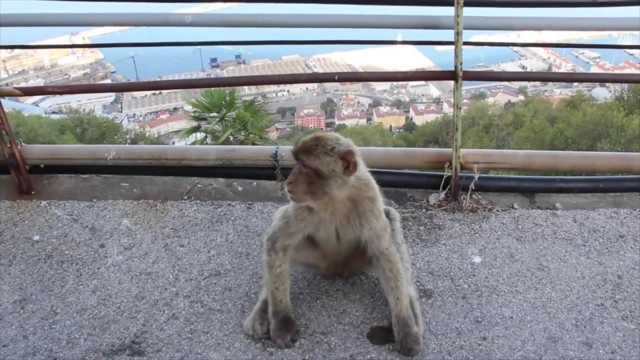 actually get into the Mediterranean through the Straits of Gibraltar. They'll tend to be slightly longer. It means that you do get to see a much more diverse amount of culture. So you'll see the Mediterranean, but you'll also get to see parts of northern France, Portugal and also Gibraltar. 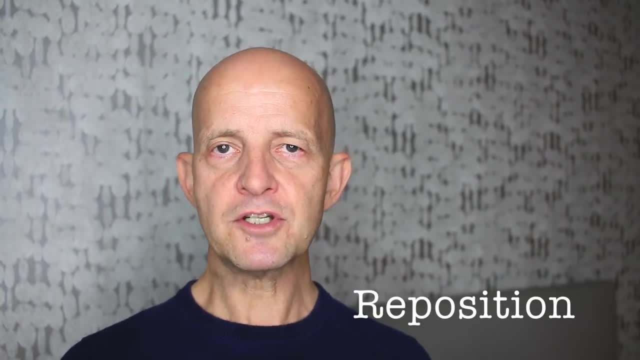 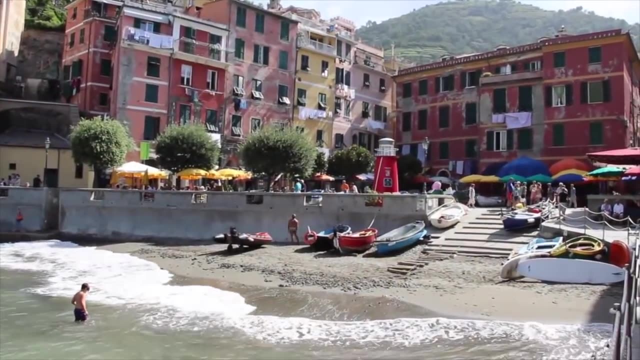 The last of the Mediterranean cruise types are the repositioning cruises. These happen at the beginning and the end of the season when the ships are normally redeploying to or from the Caribbean. So you normally see a little bit of the Mediterranean. then you will head across the Atlantic and spend a little time in the Caribbean. So that's quite a. 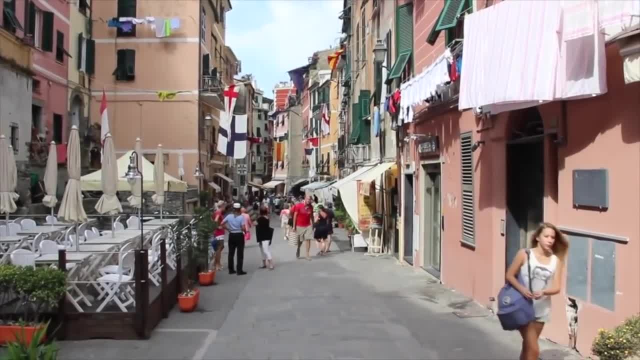 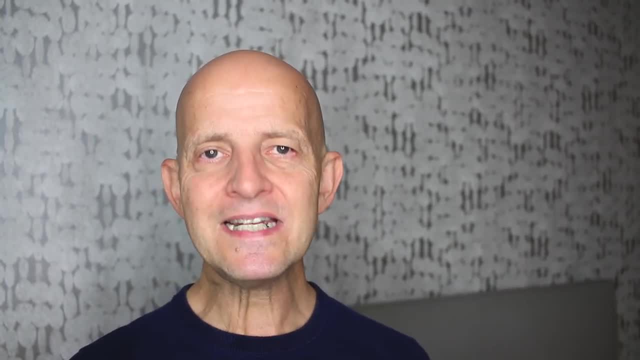 nice mix of the two regions. Now my fourth tip is a very, very important one. Make sure that if you're going on a Mediterranean cruise, you choose the right cruise line. There are at least 20 different cruise lines that will offer Mediterranean cruises during the season, So 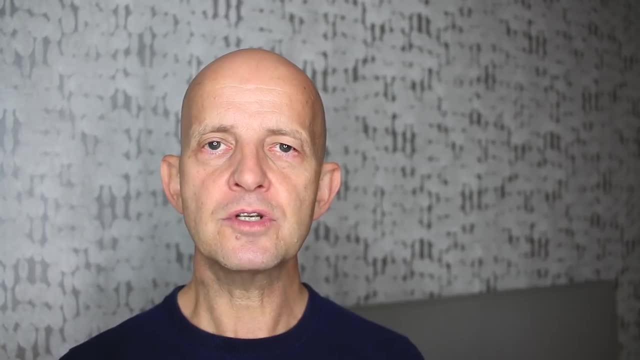 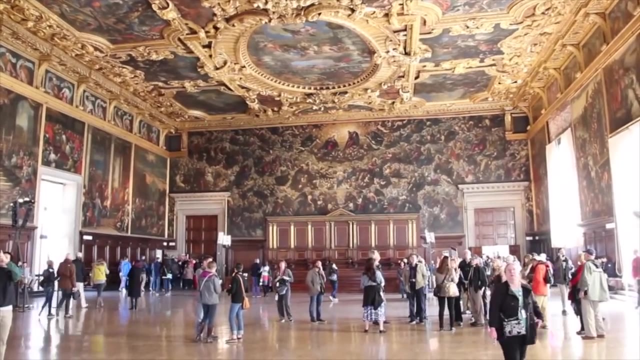 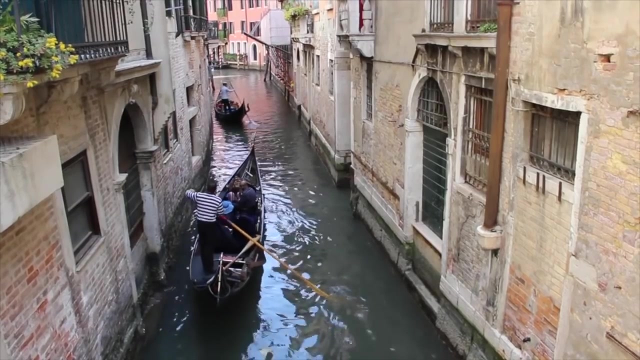 there's a huge amount of choice, and so you need to make sure that you choose a cruise line that suits your travel type, your budget and your interests, because they are very, very diverse. So, for example, travel to the Mediterranean include the following: Princess Fred Olsen, Celebrity, Aida Costa. 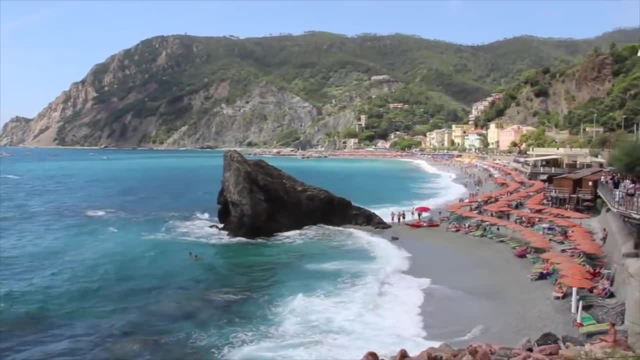 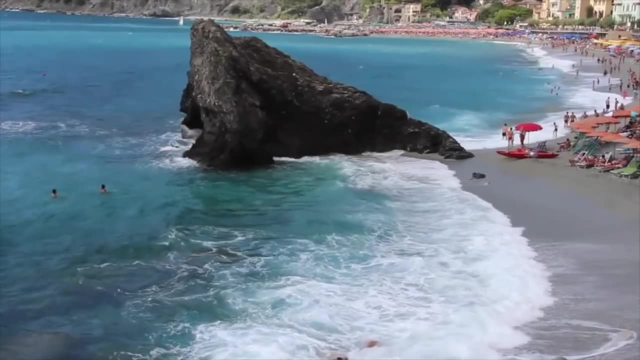 Hapag-Lloyd Silversea Region. Seventies. Saga Cunard, Royal Caribbean, Norwegian Cruise Line, Seabourn, MSC Cruises, P&O Cruises, Saga Holland American, Marella Cruises. Now, broadly speaking, 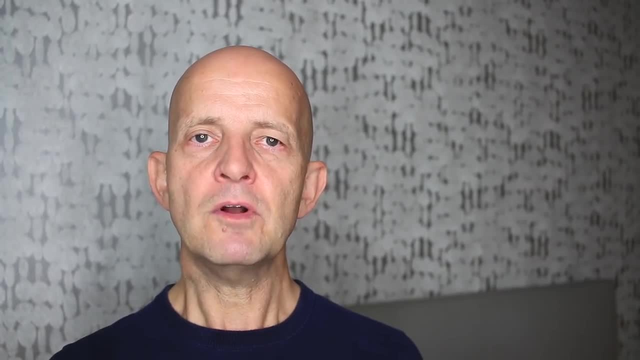 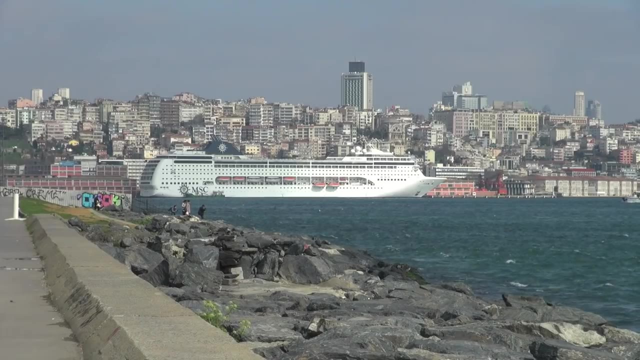 they will do the same itineraries, so it's not so much about the itinerary. Once you've decided which part of the Mediterranean you want to go, and make sure that you get on the right cruise line, because if you're on the wrong cruise line, you will not enjoy your Mediterranean cruise. 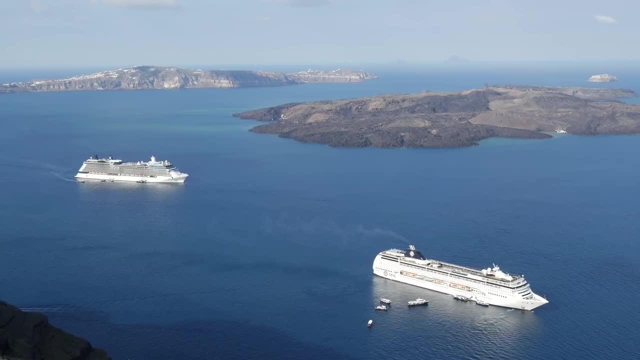 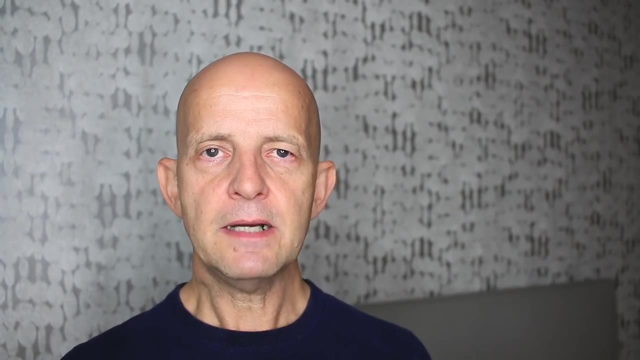 Because the passengers won't be right for you, the onboard experience won't be right for you and it's also possible the excursions won't meet your interests and needs. So, very importantly, do your research Now. linked to that, my next tip is also when you're looking at which cruise line to go. 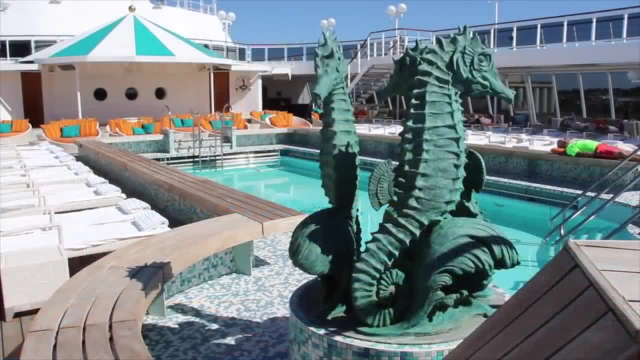 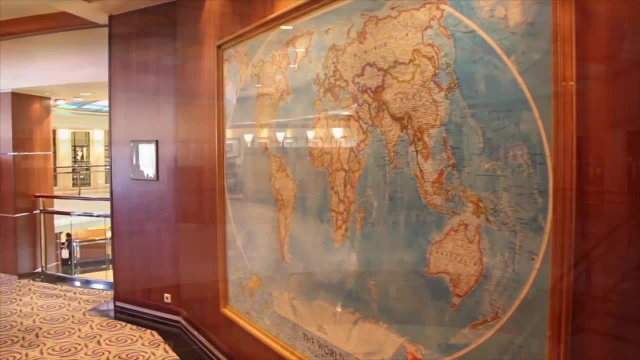 look at the size of ship. The size of the ship is important because the itineraries will differ slightly. You'll find most bigger ships are limited on the ports they can go to in the Mediterranean. These are ports that can really cater for big ships On some of the smaller ships. 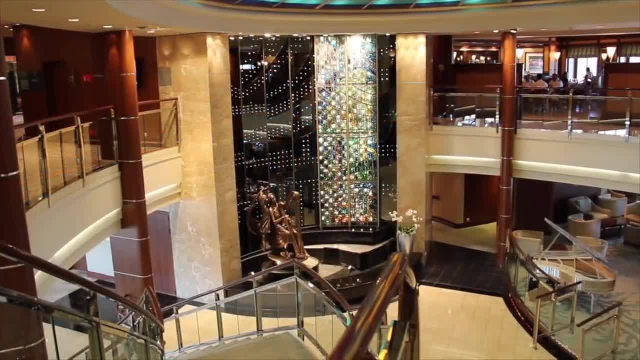 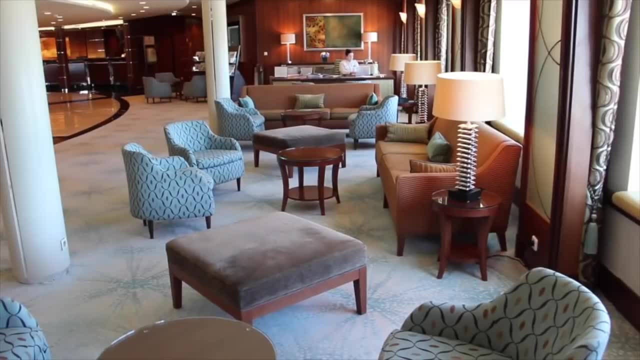 they might actually go into slightly more unusual and smaller ports. So not only choose the right cruise line, but, within that cruise line, also focus on the size of the ship and look very specifically at the ports that they go to. Now my next tip is about pre and post cruise stays, because if you're 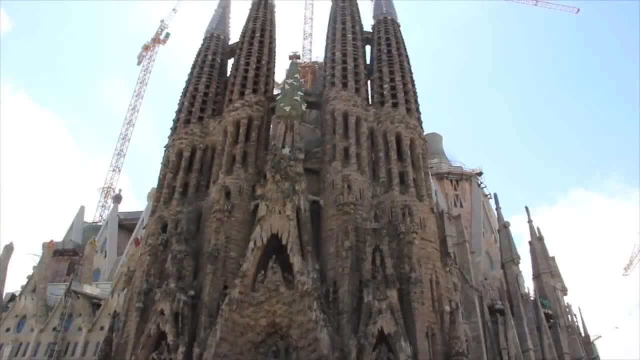 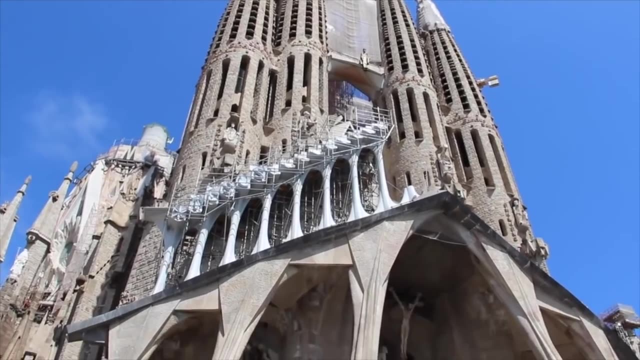 for example, sailing out of Barcelona, or you're sailing out of Venice, or even you're sailing out of Civitavecchia, which is the closest port to Rome, you're not going to get a chance to see those cities. You need to think about a pre-stay or a post-stay, based on where your cruise is. 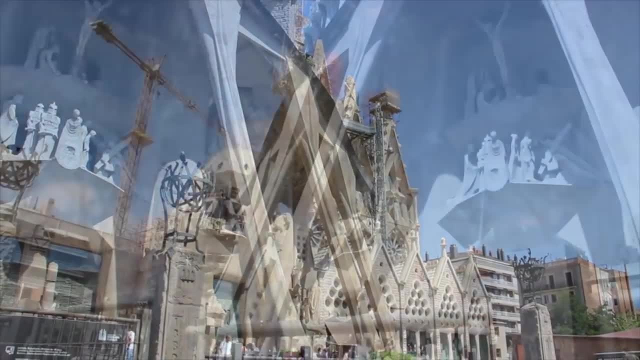 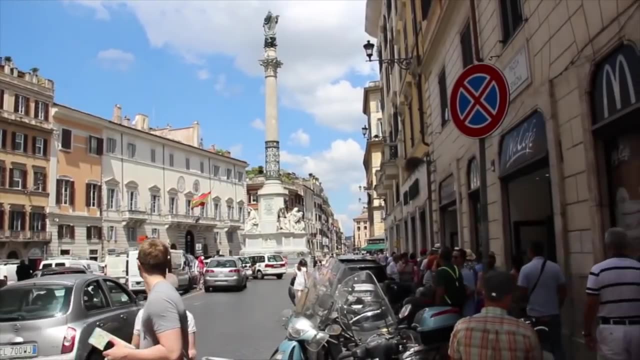 going, Otherwise you're not actually going to see those incredible cities. Now my next tip is around excursion. Obviously, if you're going on a Mediterranean cruise, you want to see the incredible sights. There's a couple of things that you do need to be aware of. First of all, some of the 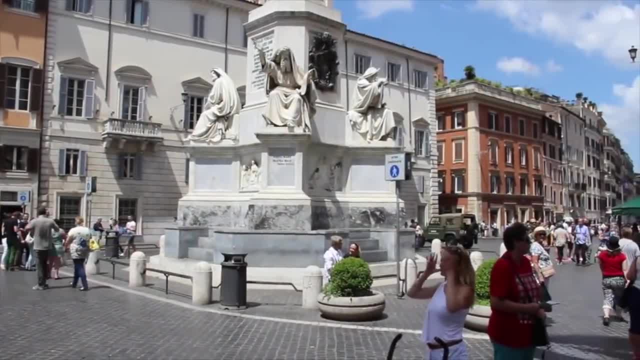 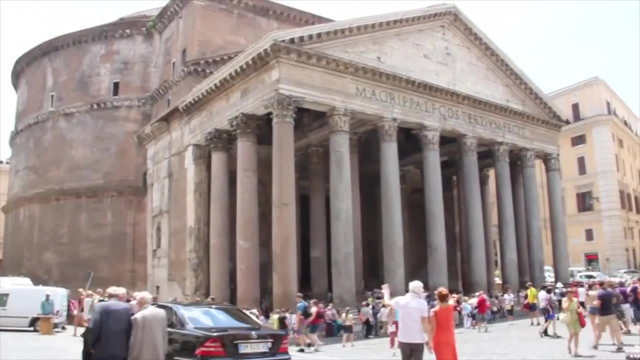 ports that you go to are actually nowhere near where it says on the itinerary. So, for example, Rome is actually a good hour and a half- two hours away from the port. You might be thinking you're going to Florence or Pisa. Again, it's going to be an hour and a half or two hours away. 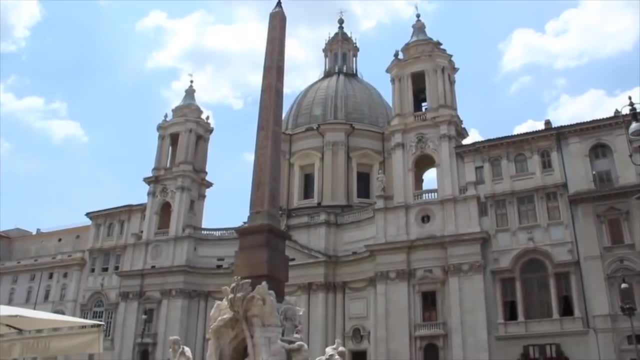 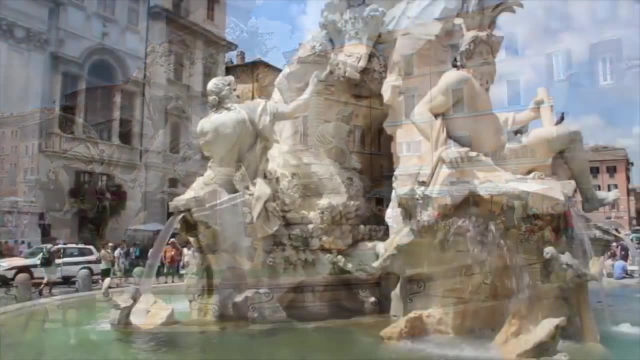 from the port where you actually dock, because you dock in Livorno. If you're actually going on one of those cruises that come from northern Europe, you might be thinking you're going to Paris, but actually Le Havre can be two or three hours away from Paris, So very. 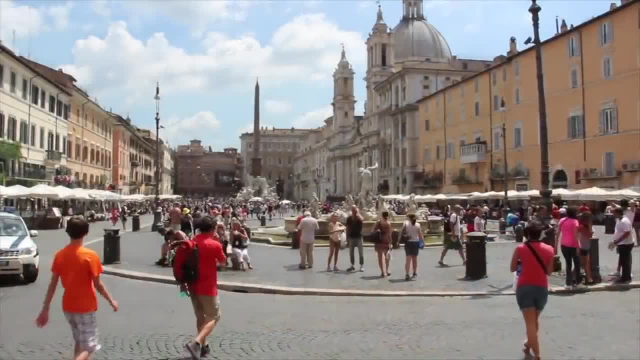 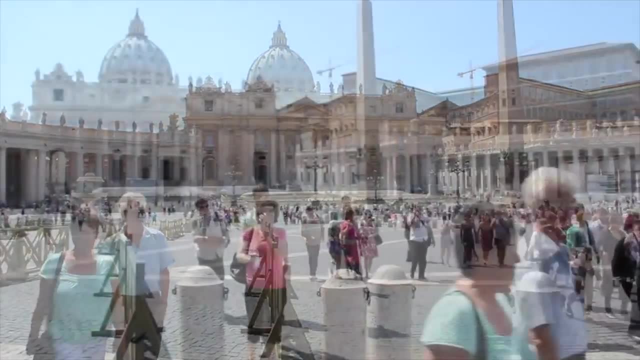 importantly, as you look at the itinerary, understand how close the actual place that it's built on your itinerary is to the port. You may want to book excursions with a cruise line because there's obviously lots of risk that you might find it difficult to get back in time before the ship. 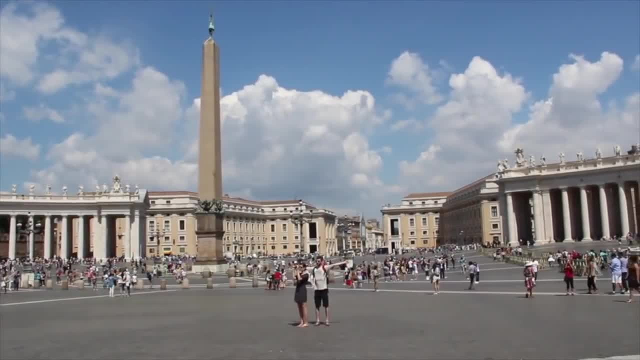 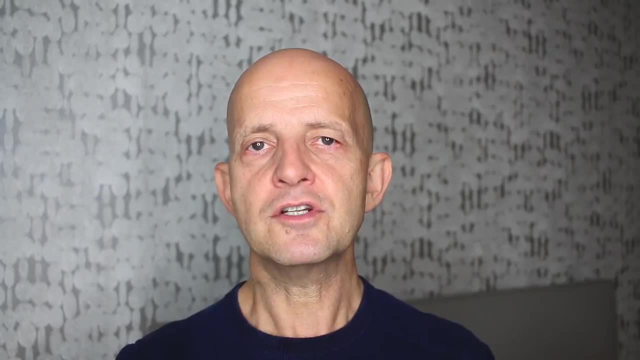 departs. If you're on a cruise line excursion, the ship will wait for you. if it's running late, If you're doing independently travel and you get to the port, you might want to book an excursion. If you're confused with the trains coming back or you miss your taxi or whatever, there's a chance. 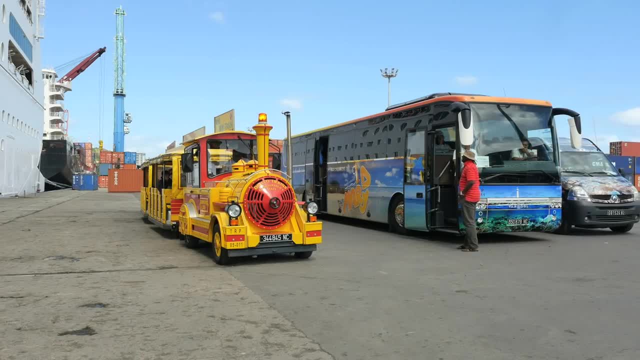 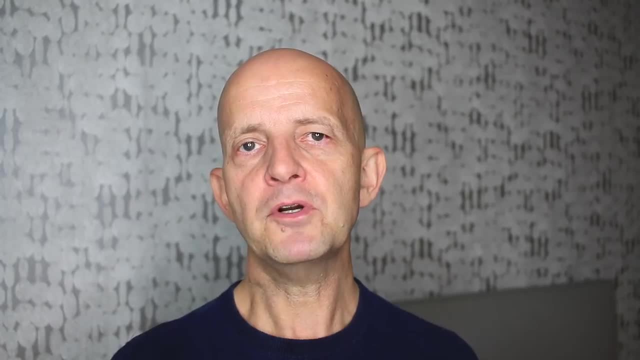 the ship will leave without you. The other thing to understand is if you are docking, as you will often do in many of the ports in Europe, you might be in a more working shipyard. often the cruise line will put on a shuttle bus service which runs you into the closest town. So if it's doing that, 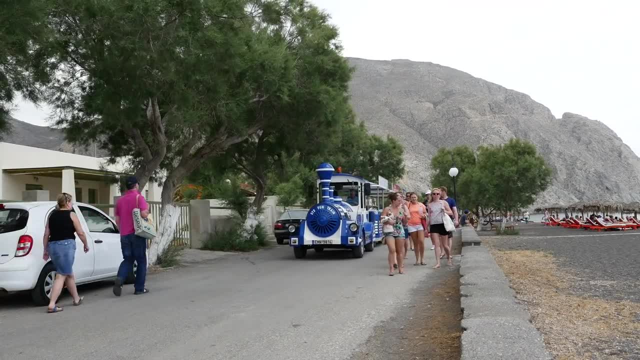 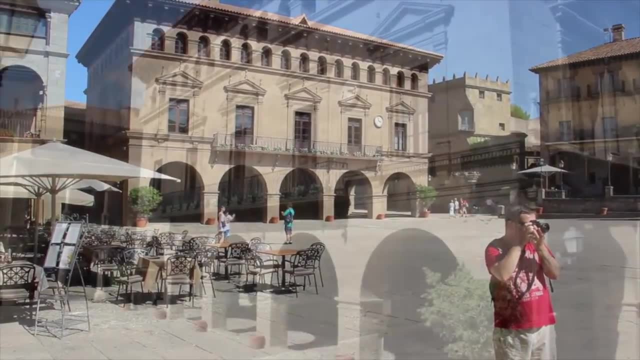 you may want to consider actually self-touring in those particular ports, because many of them will have hop on up with buses, or there will be talks on board, or there'll be materials given on board, or the tourist board will either be on the quayside or come on the ship to let you know how. 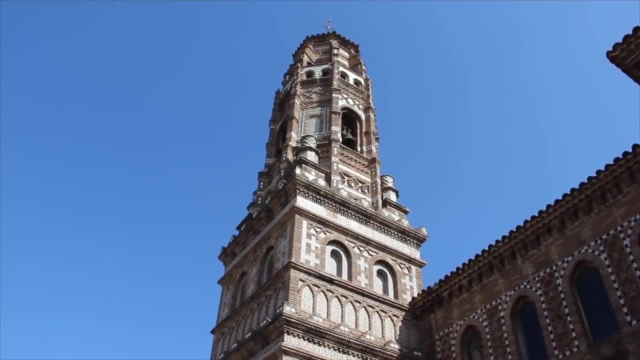 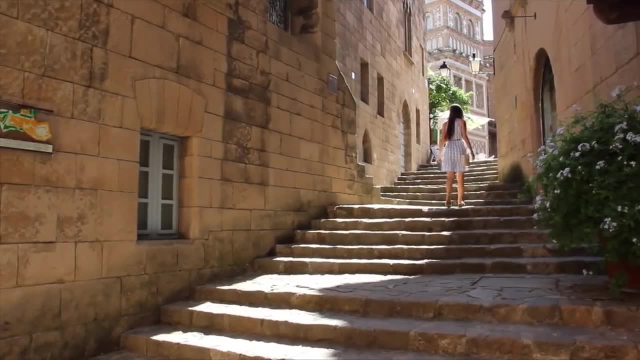 you can self-explore, So you may, in those spots, want to consider doing some self-exploring. Very important you want to understand in each of the destinations and ports you're calling out is just how close the sites or place you want to see is to where the ship is going to be, and then plan your. 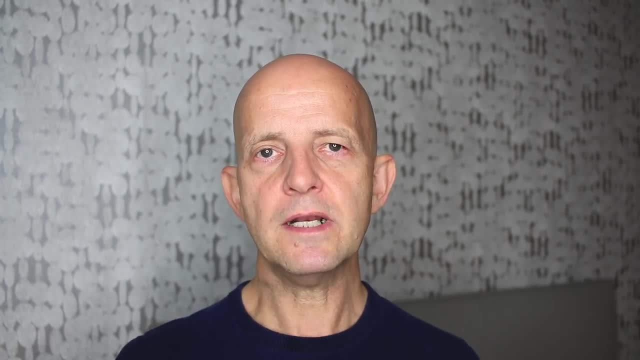 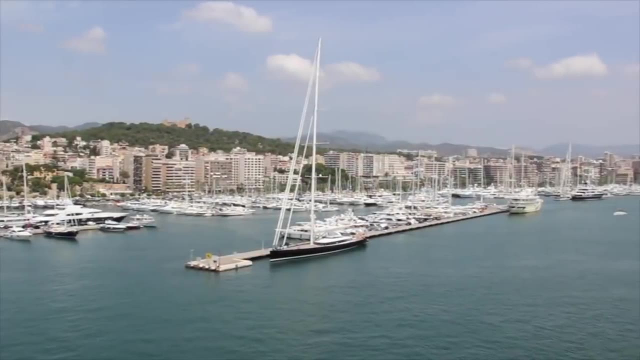 excursions once you understand that. Now my next tip is also linked to that- is: if you're on a European cruise, there is a lot to see, a lot to do, so don't over schedule. One of the things I recommend is, as you look at the itinerary, because you're probably going to be on a cruise and you're 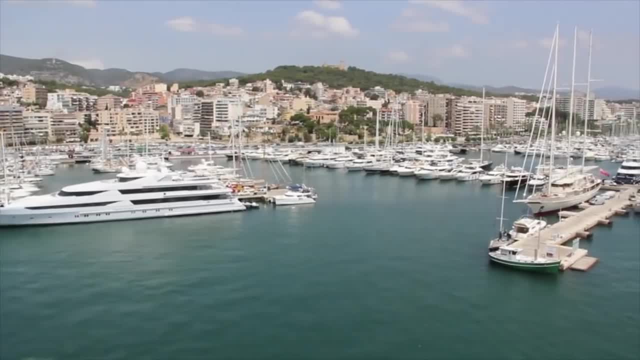 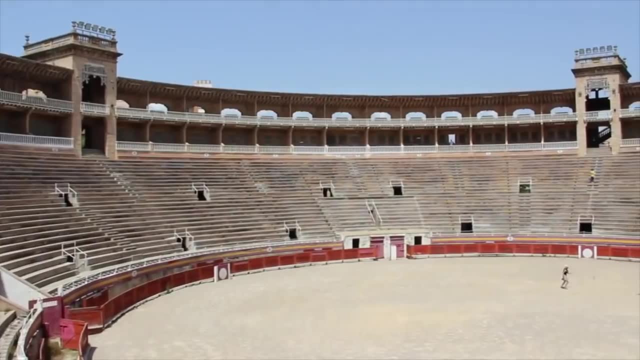 in a port every single day is perhaps think about having a mix of self-touring and excursions, because it could be very tiring if every single day you're up early, you're out touring all day, because some of these will be all-day tours, all-day excursions. Pick a day or two where you're. 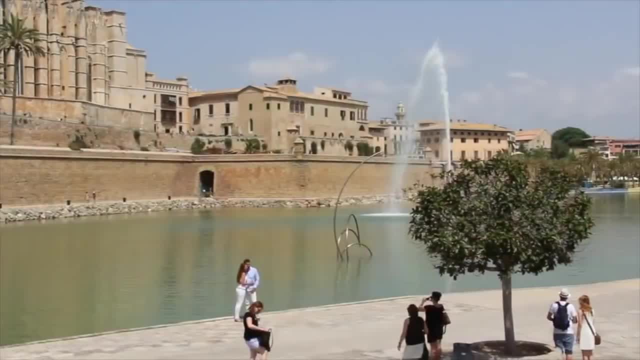 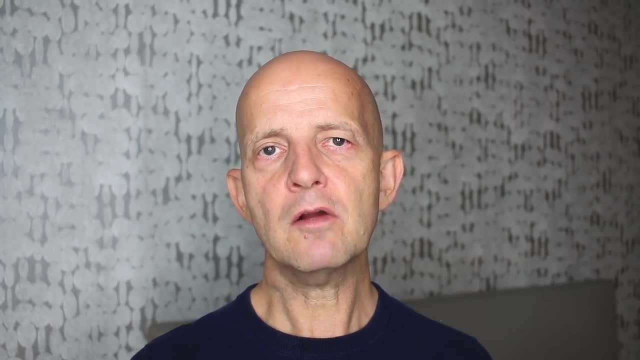 going to be quite close to the town, do a bit of self-exploring, have some time just to sit in a cafe, watch the world go by meander around, perhaps sit on the beach. The other thing you might want to think about is your dining time. So if you're going on one of those cruises which has 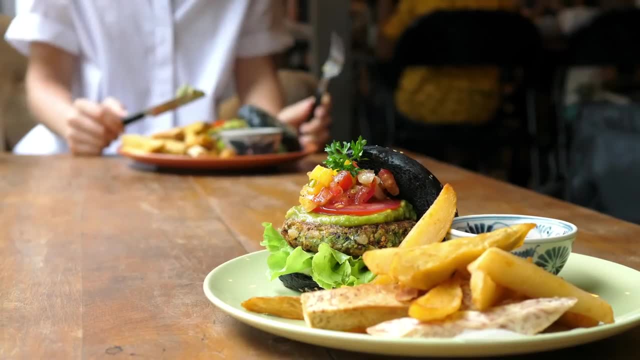 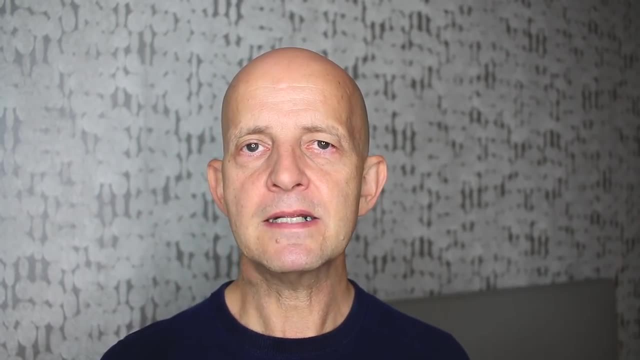 fixed dining times. you have an early sitting and a late sitting. now, if you go on a Mediterranean cruise, you're likely to find that many of the excursions will be quite long, so you'll be out all day. So one of the things you might want to think about is: 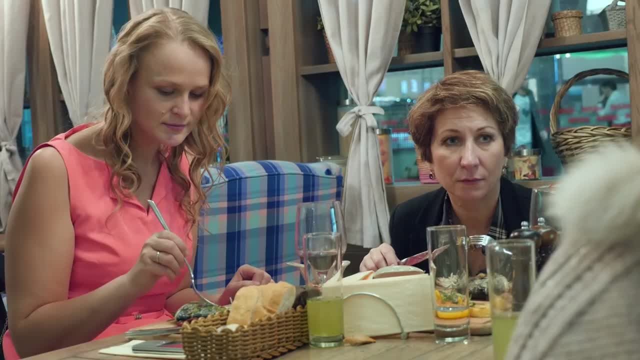 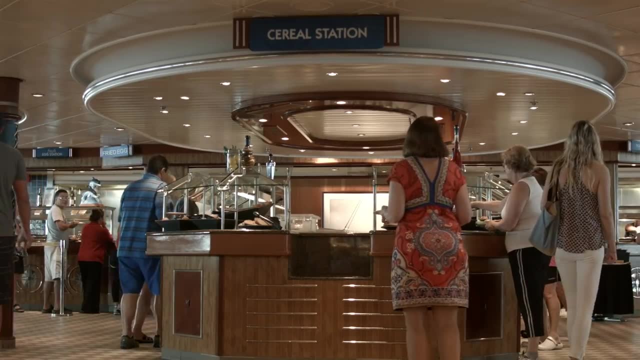 actually, if you do have to choose a first or second sitting is consider the second sitting because it's going to give you time to unwind, get ready, chat about the day and then go to the later sitting. It may give you a less frantic overall Mediterranean trip. The other thing to 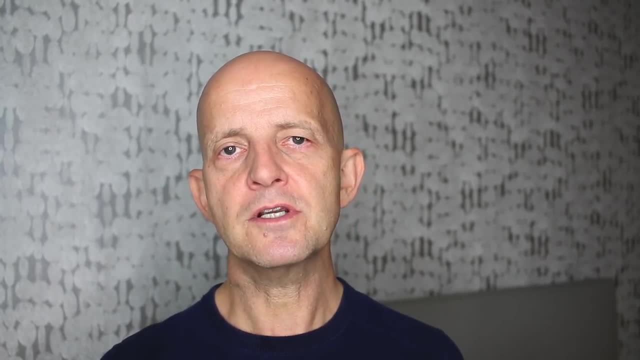 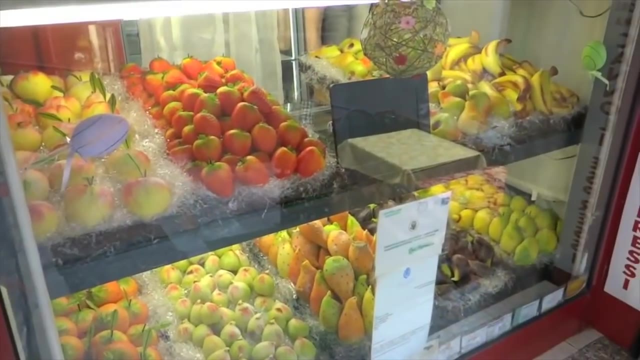 think about is currency. Now, on a Mediterranean cruise, most of the places you're going to go to are going to either be Euro countries or you're going to find most of the tourist places that you interact with will accept the Euro, So probably the currency you need for when you're on on land. 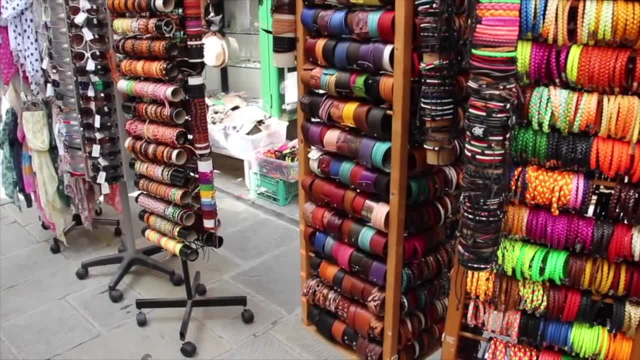 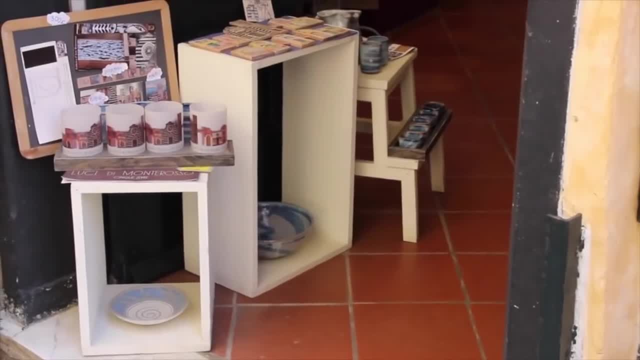 is the Euro. You'll find pretty much every place. certainly the cruise line will take you. they're used to taking Euros. I wouldn't worry too much about taking different currencies if you're going to places that are not Euro countries. Now, when you go on a Mediterranean cruise, one of 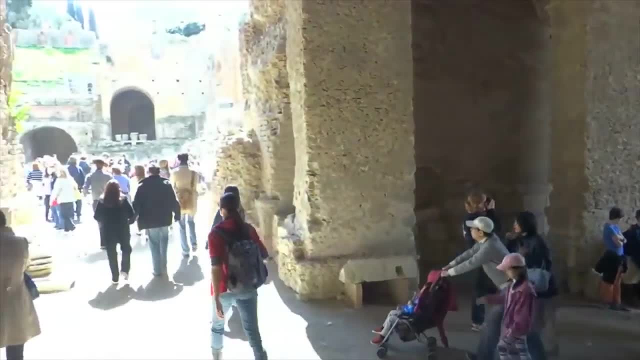 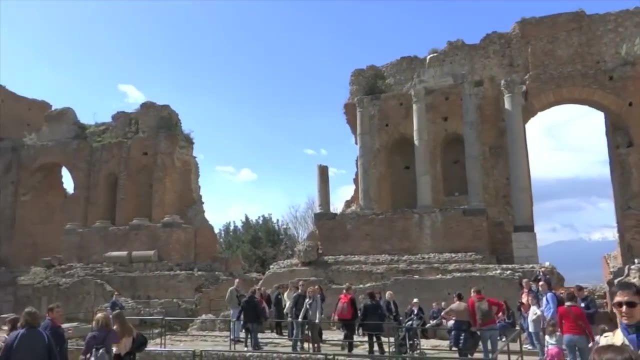 the things I recommend you do is see it as a taster for understanding Europe, understanding the places you may want to go back and explore. So if you're going to a Mediterranean cruise, you're going to visit lots of places, you're going to see lots of different countries. 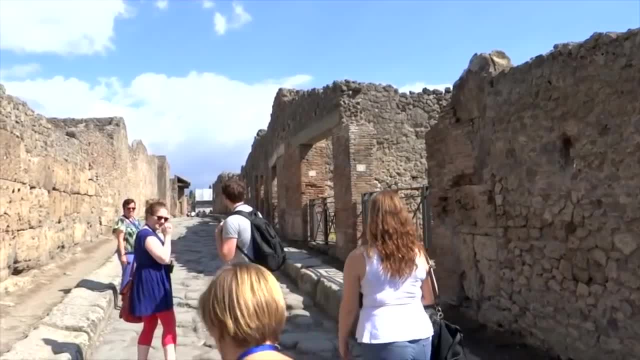 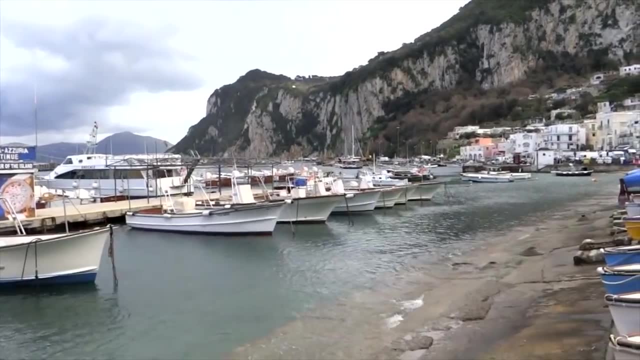 lots of different sites. You're not really going to understand and see Europe in a huge amount of detail, but it's going to give you a feel and a flavour for that place. Go with your eyes open and think about. perhaps your plan is to come back and explore much more on land and get a little bit. 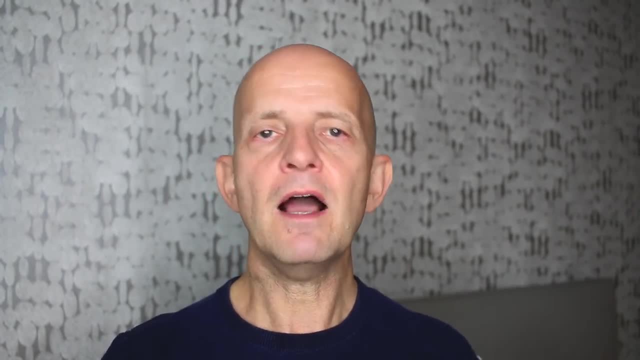 deeper. A Mediterranean cruise is fantastic. There are five different types of ways of seeing the Mediterranean, as I've explained in the different itineraries, but you're going to get a chance to immerse, feel and explore the world. If you're going to a Mediterranean cruise, you're going to 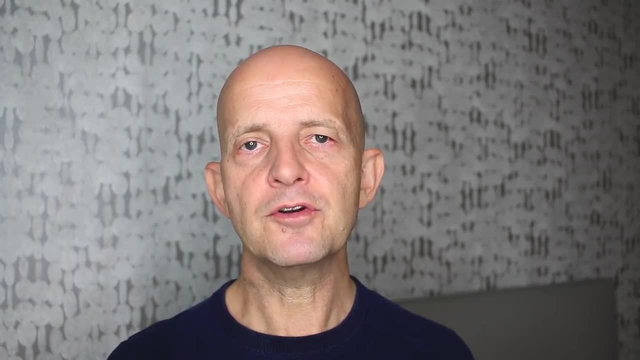 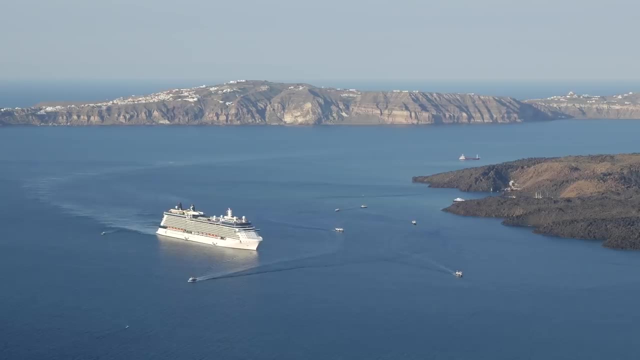 feel and get a real taste for Europe. It's great a Mediterranean cruise because in the space of a week or two weeks you're going to see lots of different countries, lots of different cultures, experience, lots of different sites. A cruise is really a great way of seeing the Mediterranean. 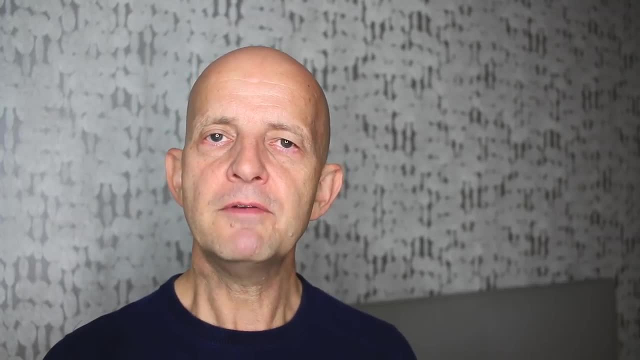 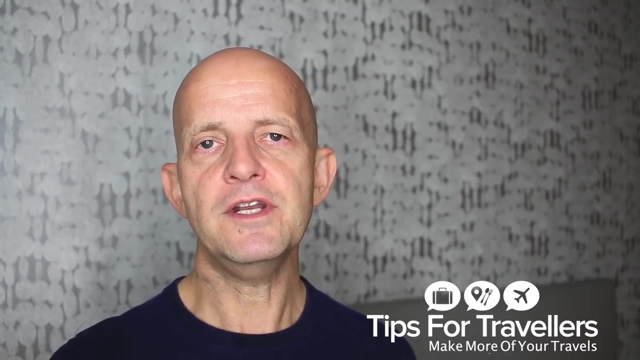 If you enjoyed it. I'd love it if you gave the video a like and a thumbs up, but, very importantly, please subscribe to Tips For Travellers because you'll get much more travel inspiration, advice and tips every single week as a new video is posted on the channel. 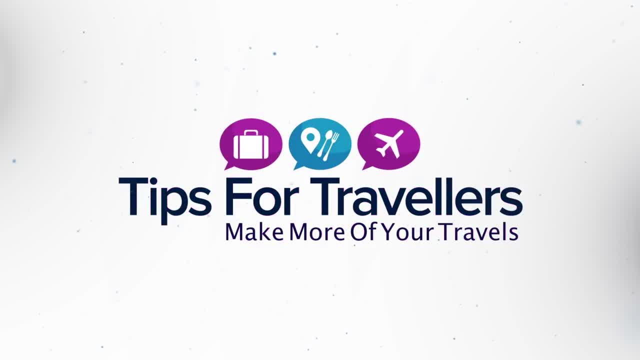 I'll see you in the next one. 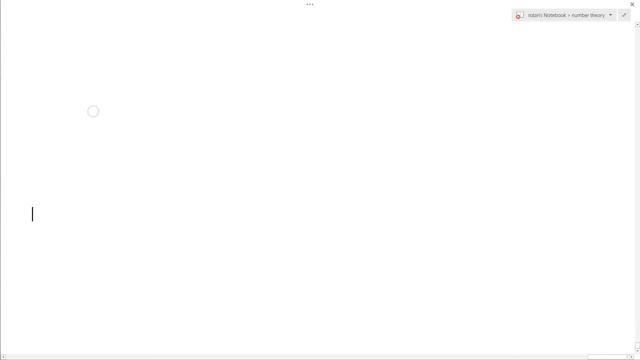 Okay. so we've got another multiplicative function I'm going to talk about. I'm going to talk about the sigma, oops, the sigma. Okay. so last time we talked about multiplicative function, Multiplicative functions. Just to remind you, m? n greatest common divisor equals 1,.